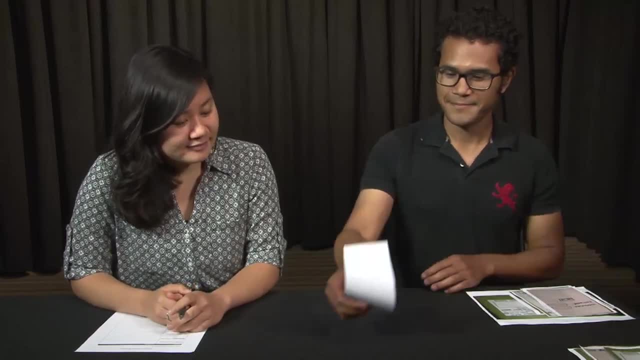 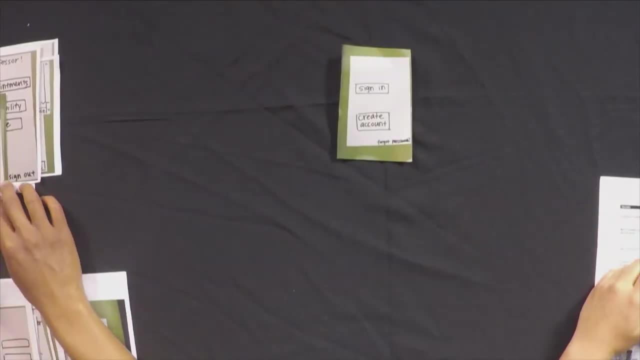 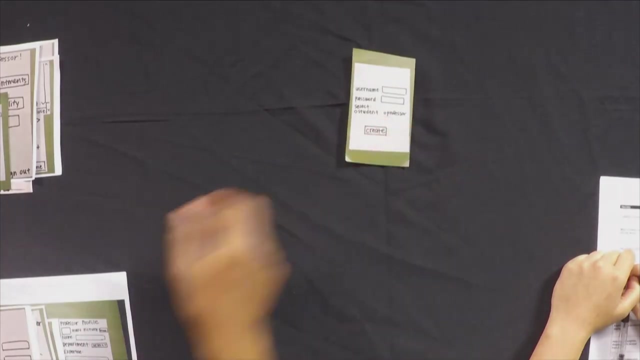 So let's get started. So this is the first screen, and I don't even know what prototype I'm testing because there's no name on it, So I'll just create an account. So here I'm going to make a username and password, I'm going to pretend to be a professor and click create. 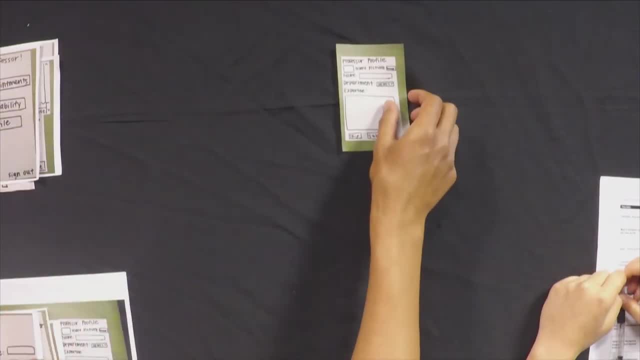 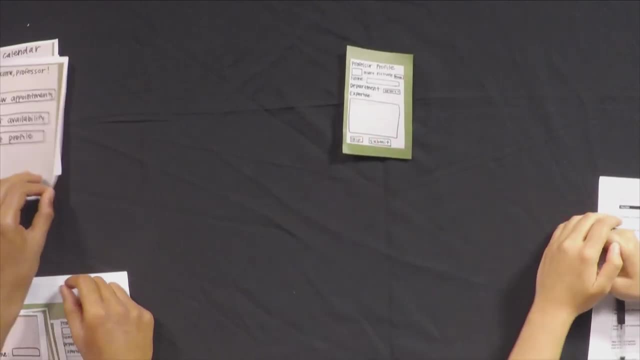 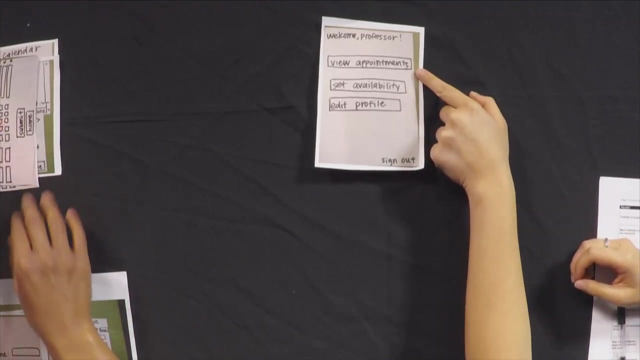 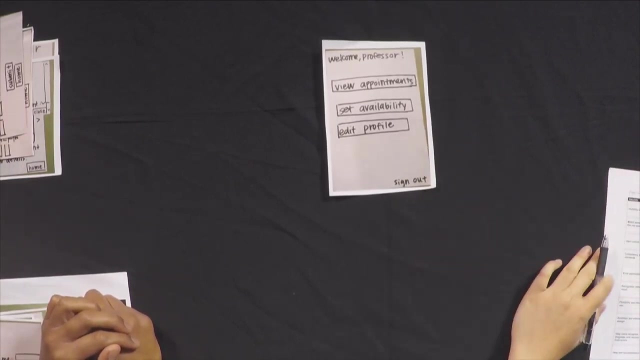 I'll fill out my name and then I don't want to set up my profile, so I'll just click skip. Here's the home screen. It looks like I can view appointments, set availability or edit my profile. What if I want to view my profile? It looks like there's no way to view my profile. 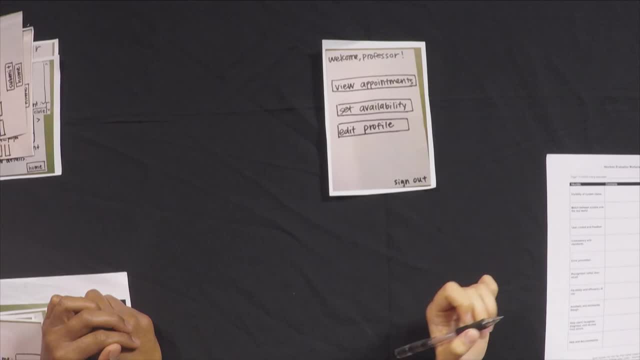 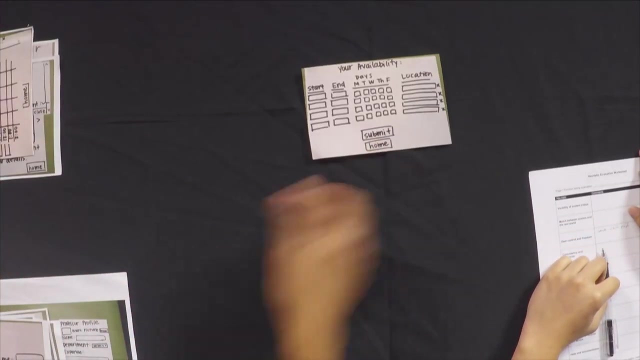 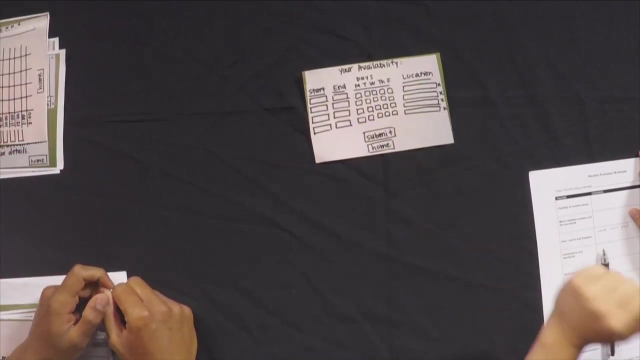 So I'm going to put that down as a problem. And here you can see that I have user control, Can't view profile, And I'm just going to set availability first. Here I see there's start and end times And I can check some days of the week and add a location. I think there are a few problems here. 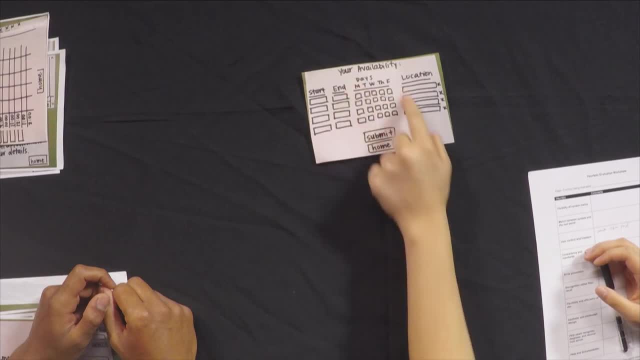 So I noticed that the one- there's only days of the week, but they don't tell you which day it is- is I think the actual date is very important. and two, I think there's an issue of flexibility and efficiency of use, because if I were a professor and I 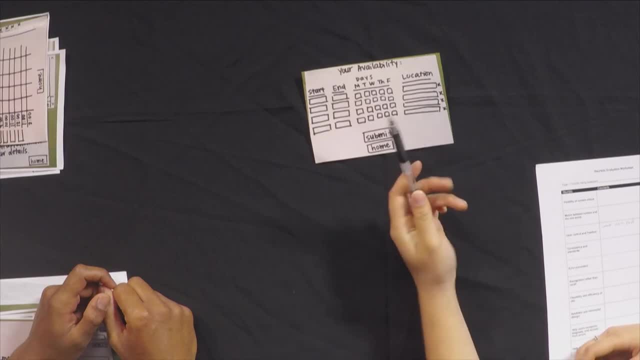 use this a few times, I think. usually I would meet in the same locations and I wouldn't want to fill this out every time, so I think there should be a faster way to go through this process, so I think I'll put down: advanced users function under flexibility and efficiency of use, so let's submit some. 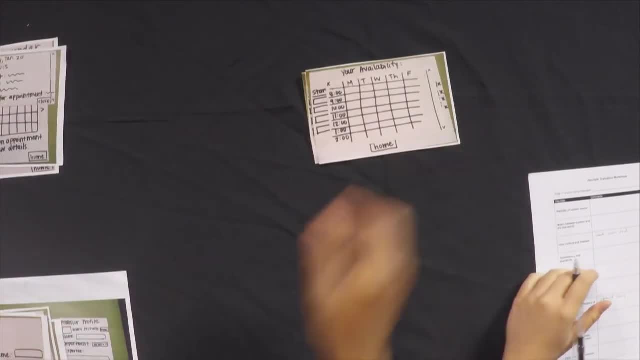 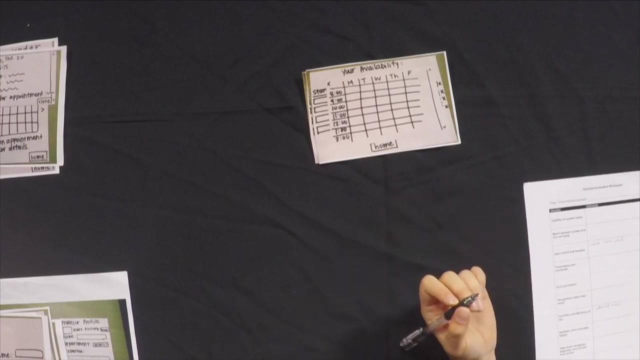 times. oh, so here are all my available times that I set. it would have been really nice if I was able to see this before setting some times. you, but that didn't seem like it was available, so I'll add this to visibility of system status that I should be able to see the times beforehand. now let's. 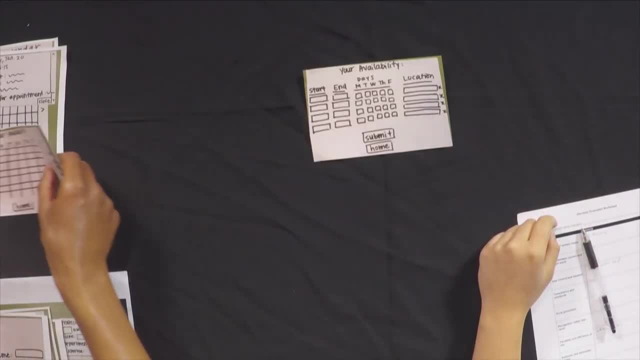 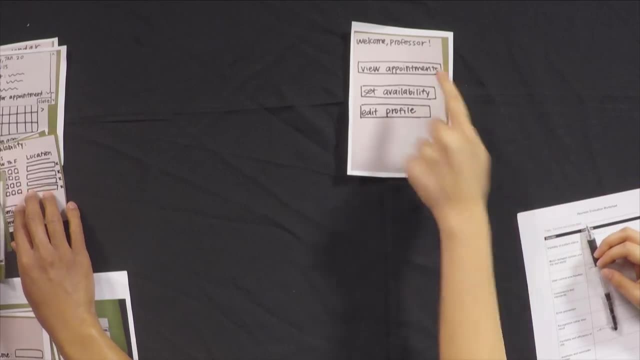 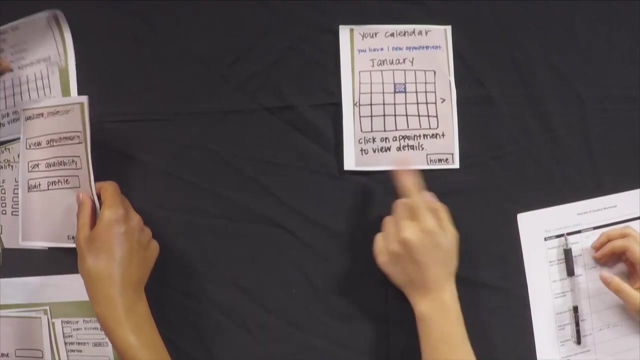 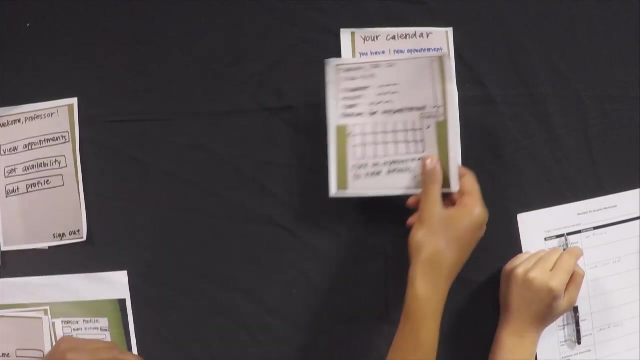 close this and let's go home. so let's, let's view my appointments now. so it says: click on a point, click on a point. click on a point to view detail details. so I'm guessing this is my appointment. click this. okay. so I have an appointment Tuesday, January 20th, with some student. 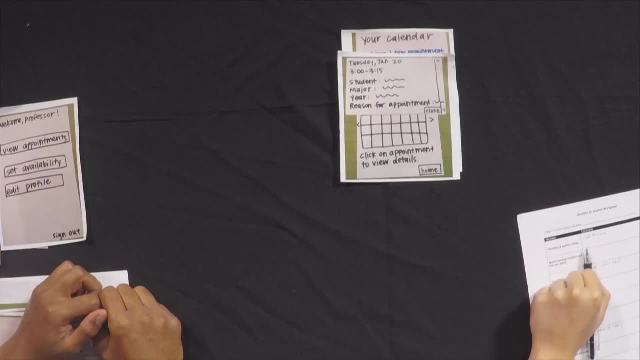 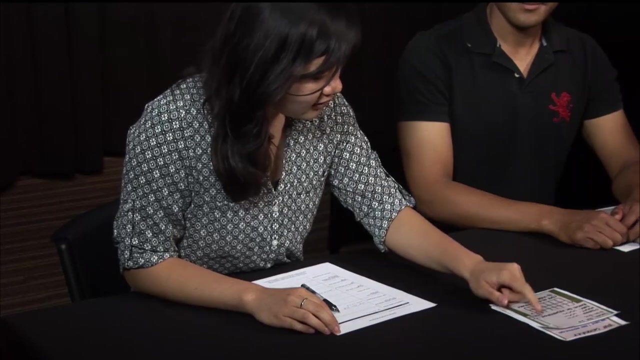 what if I can't make that time anymore? it doesn't look like there's a way for me to cancel it. I'll note that down under user control can't cancel, so I'm good. okay, yes, so now I'm just gonna look at my profile to see which accounts do. 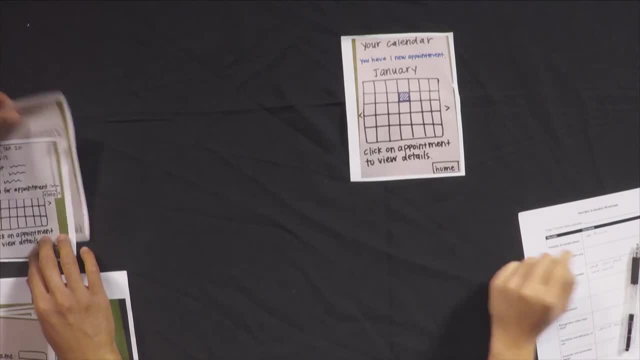 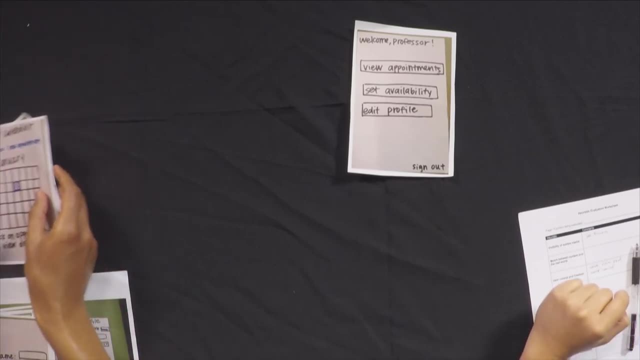 hit and load. in the next time I close this, I clear my profile and I'll just sign out. okay, so I'll check out the student side of this profile. so let me know how you're doing. um, at the endShe said about how the student is doing. 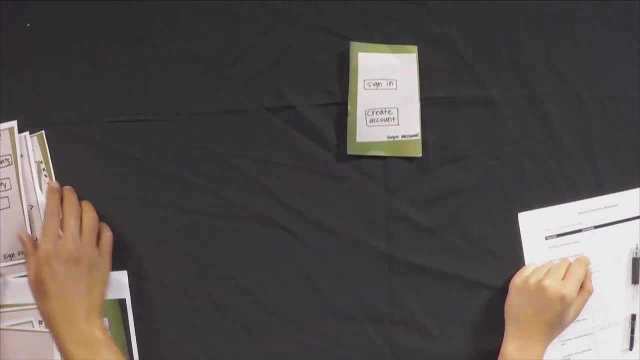 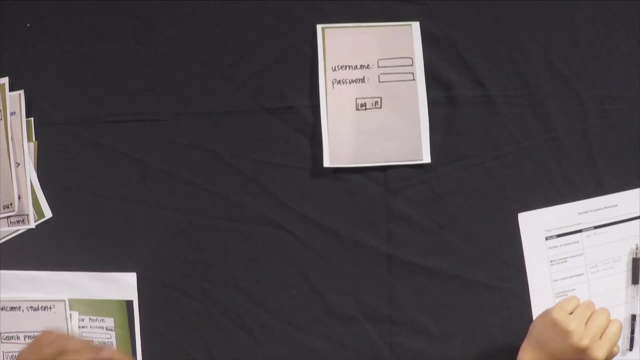 learningousing something about skills. so it may be too extensive- a lot of science. so I'll check out that and tell you how it's going to perform and if I go working I'll just hit that guard or whatever to see if that'll be helpful insidetrain. so I think I'm gonna go ahead and network and log my accounts. the 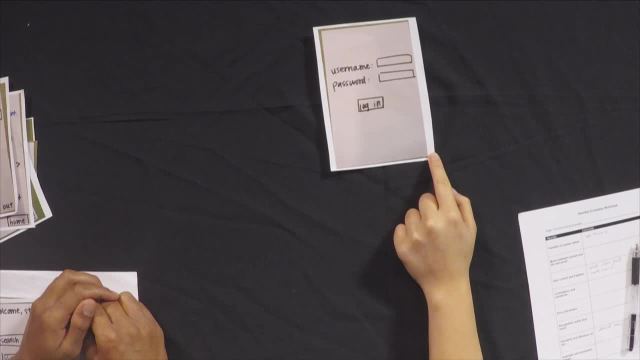 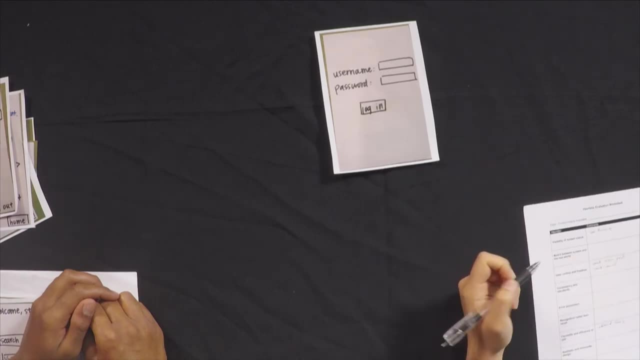 card isn't necessarily too visible and I hope you want to make that work. okay. I would definitely here on the previous screen, but it's not here anymore and also there's no username forgot username screen. i think that would go under error prevention if someone forgets their username. 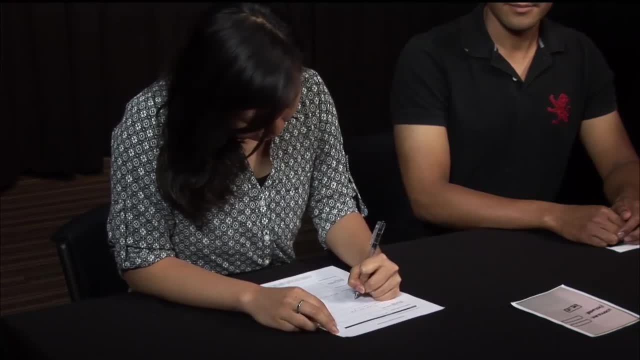 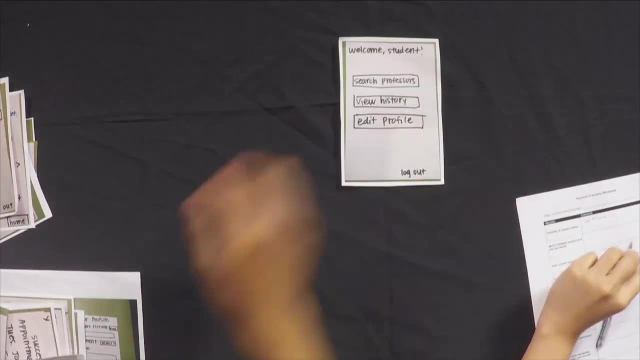 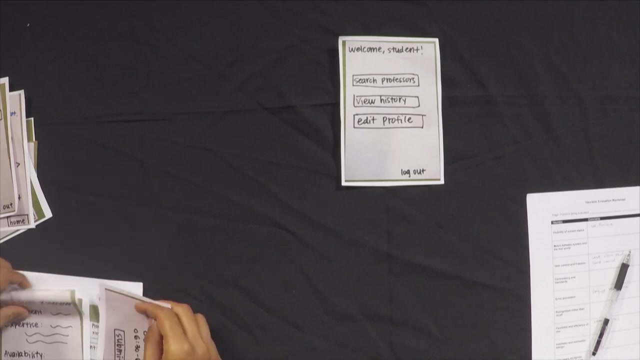 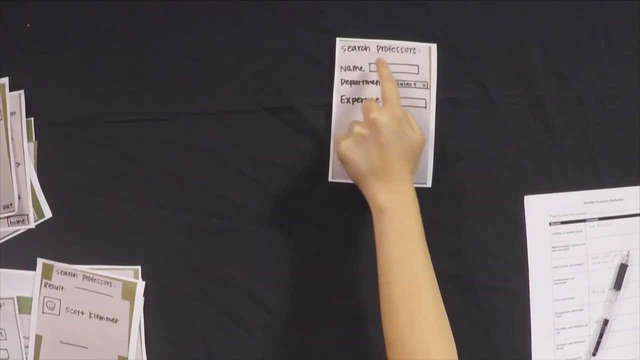 this prototype isn't able to account for it, so forgot username, so let's sign in. all right, so here, um, i want to make a, an appointment with a professor, so i'll search for the professor that i want. uh, let's see, i'll just add the name. uh, scott clemmer. 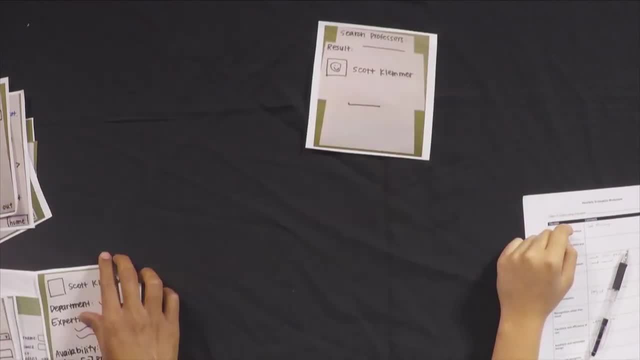 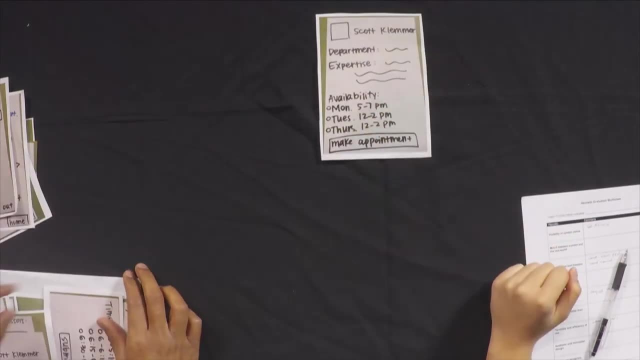 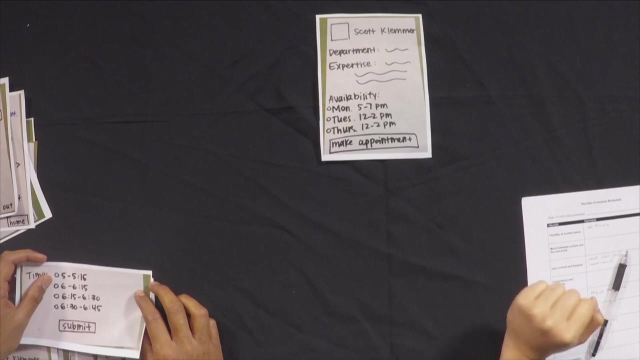 oh, and i found. i found scott clemmer, so i'll click on that, let's see. so this is his profile. um, actually, if i didn't want to make an appointment, an appointment with him, it looks like there's no way to go back or to cancel. 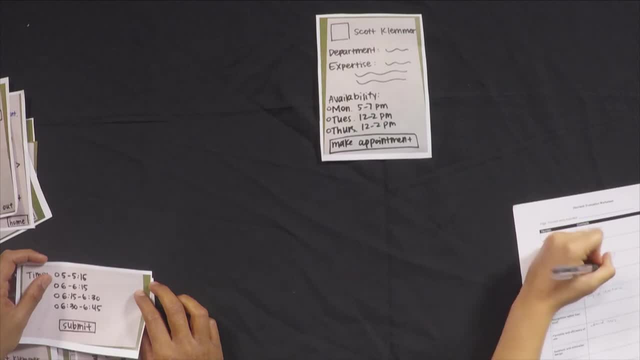 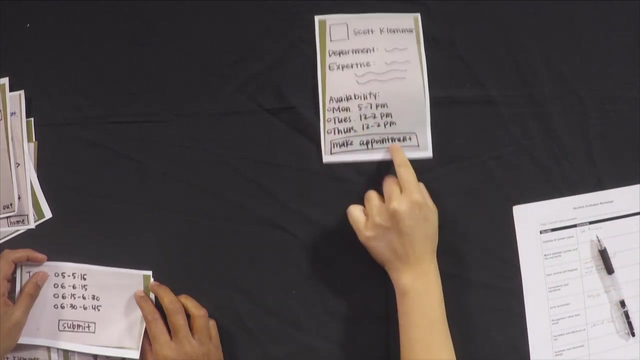 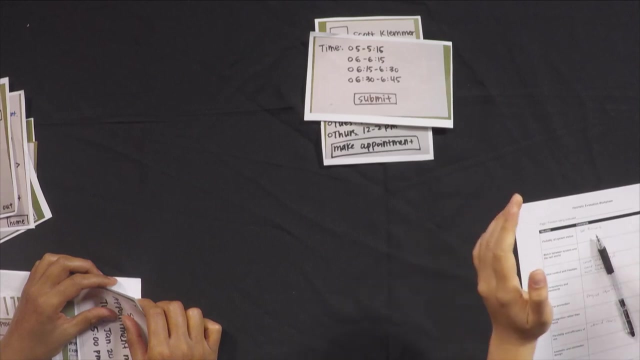 so that's another problem of user control and freedom, that i must make an appointment now. so i guess i'll make an appointment for monday 5 to 7 pm and make appointment. oh, so it looks like, uh, in the time range of 5 to 7 pm i have to choose a 15 minute time slot. 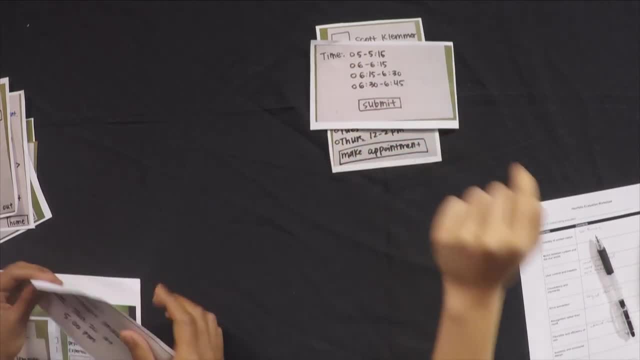 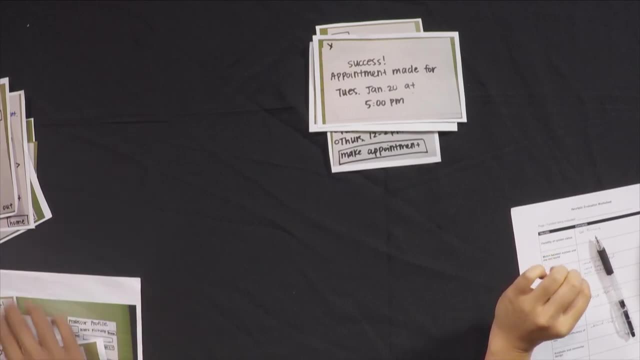 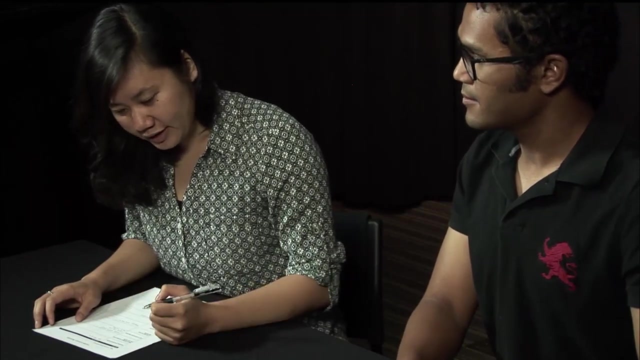 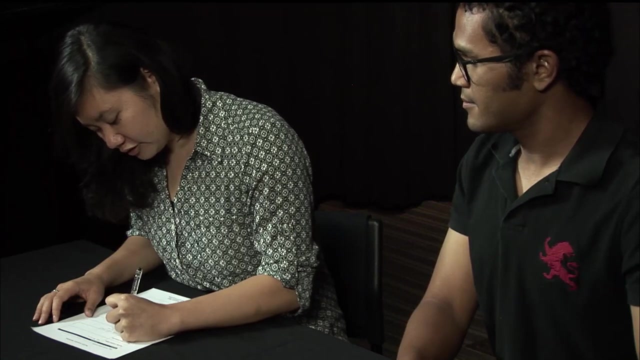 so i'll choose 5 to 5, 15 and hit submit success. appointment made for tuesday, january 20th, at 5 pm. i thought i clicked monday. um, this must be a minor error. um, just in writing, but i'll just note that down under consistency and standards. uh, monday change to tuesday. 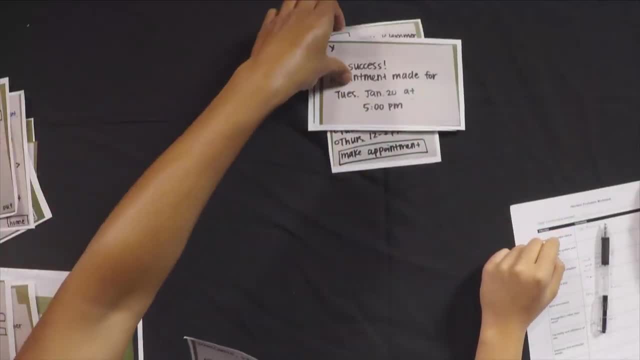 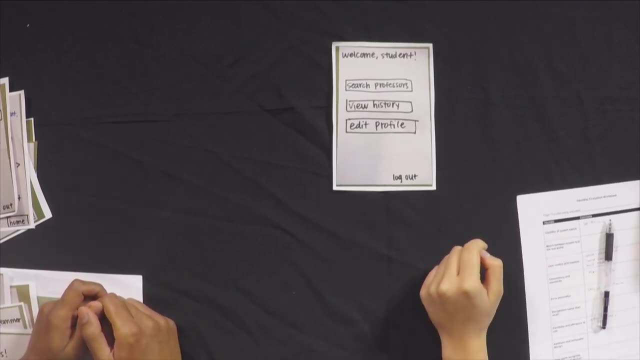 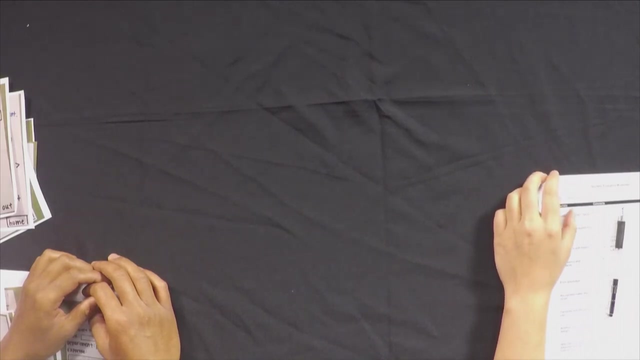 all right, so let's close this. well, i think let's just end it here- and i have some general comments about the prototype. so one thing i noticed was that there was very little help documentation in the prototype. so there was one screen that i really liked in the prototype. it was the screen where the image of the 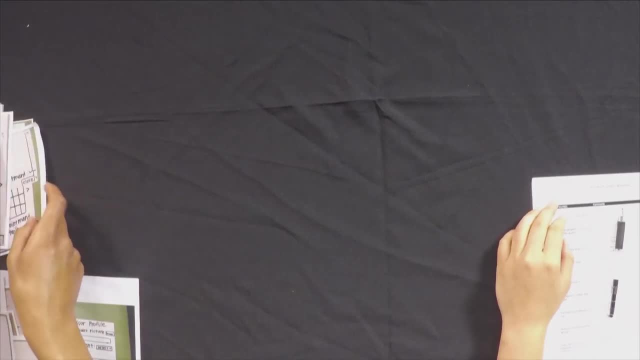 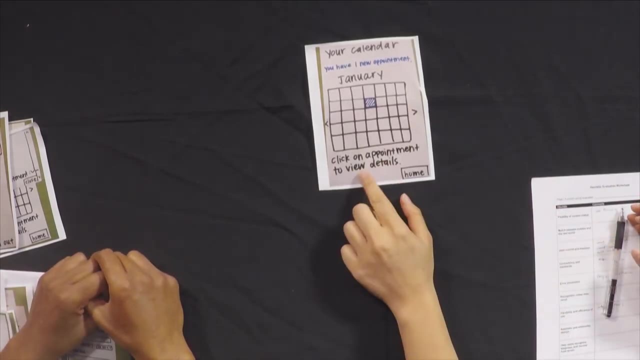 liked it was the one with a calendar on it for professors, so this one was the only one that had any sort of instructions or help for me. it says click on appointment to view details, but for the rest of the prototype it doesn't really give me any information on how to go about using the prototype. I think it 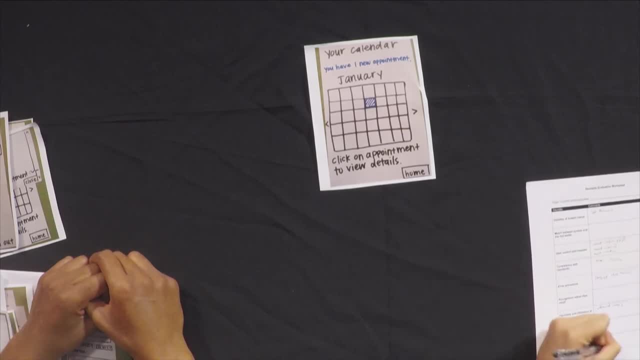 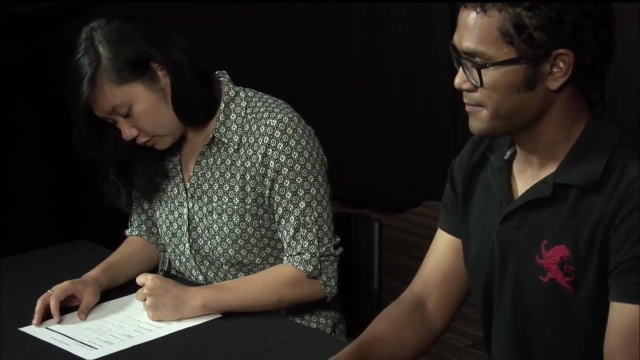 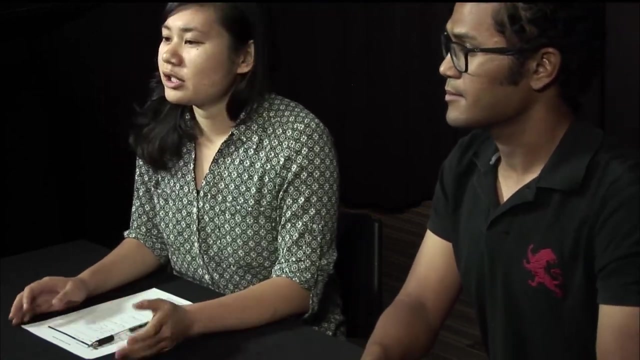 would have been really helpful to add a little bit more of that. so I'll just note that down in help and documentation need more help. so the other thing I noticed was that a lot of the prototype pages look very different from one another, so this would make it really difficult for me to remember what 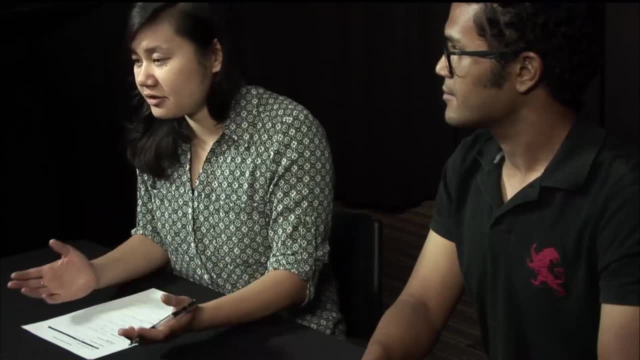 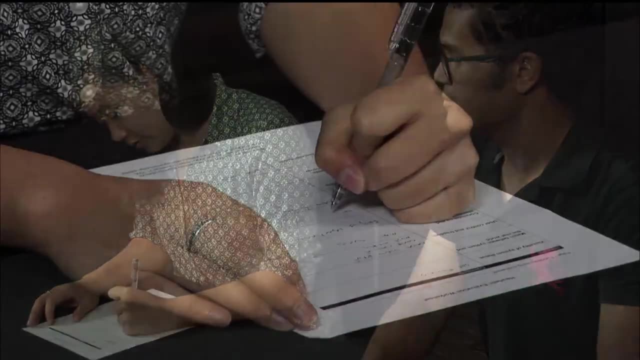 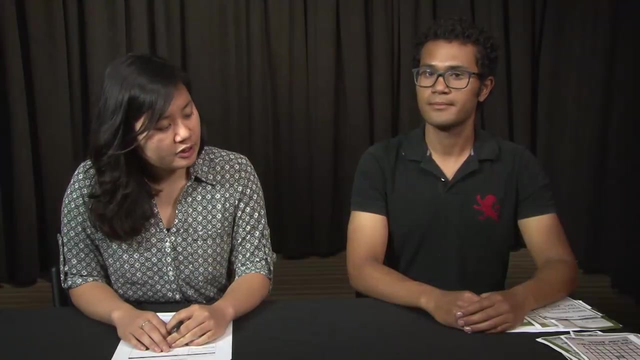 page I'm on or how to continue using it because they look so different. I think I'll write that down as a problem in recognition rather than recall. the pages are too different, too different. I think one thing that was really good about the prototype was that the match between the system and the real world seemed pretty good to me.